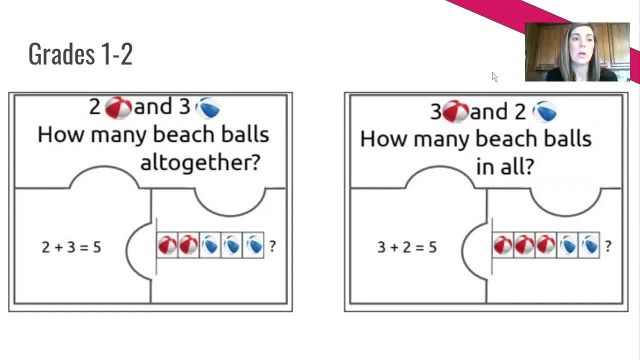 visuals in our tape diagrams and in our problems. So two red balls and three blue balls, How many beach balls all together? So in our visual model down there in the right hand side of that puzzle you can see I have put two red balls and three blue balls. That's going to really help the 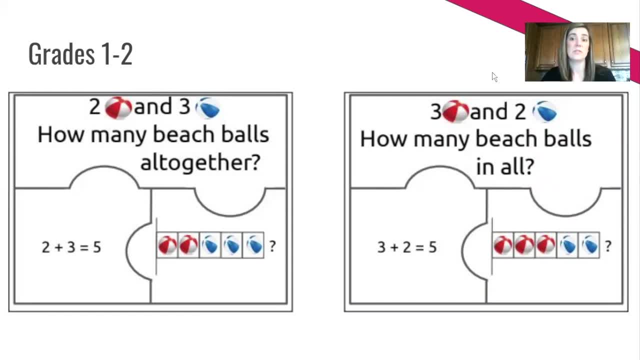 kids start to understand how we can build these visual models together. There are six puzzles that go with these beach balls. They deal with the numbers two, three and five, So they can't just match up the numbers and put the puzzles together. They really have to have an understanding. 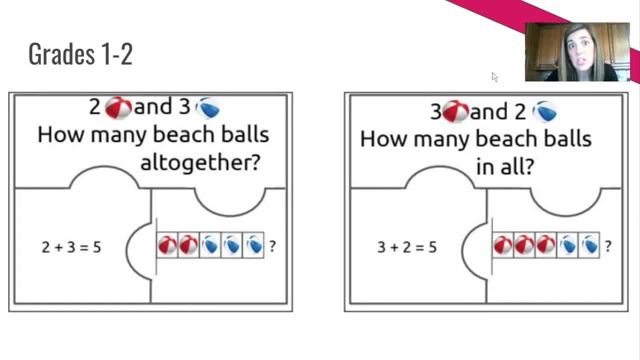 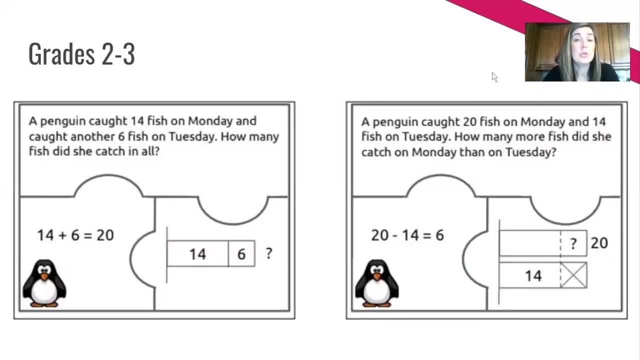 of? what is the problem telling you, What's the problem asking you? What is that equation going to be And what is the visual model going to be In grades two and three is this penguin set of puzzles. So the penguins are dealing with fish. 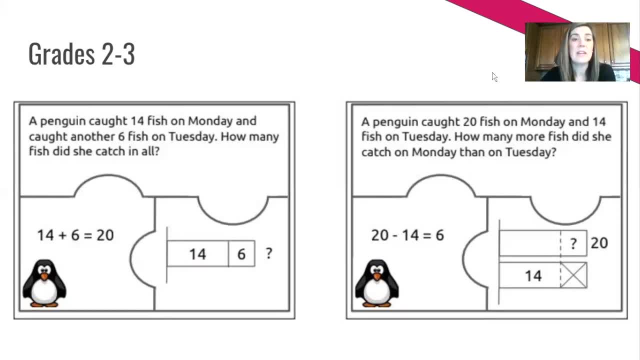 And you can see, in these two- the one on the left is a little bit more basic, We have part, part, whole, And the one on the right is a comparison problem. Kids in second, third, fourth, fifth grade need to be working on all kinds of puzzles: Part, part, whole, Or we know. 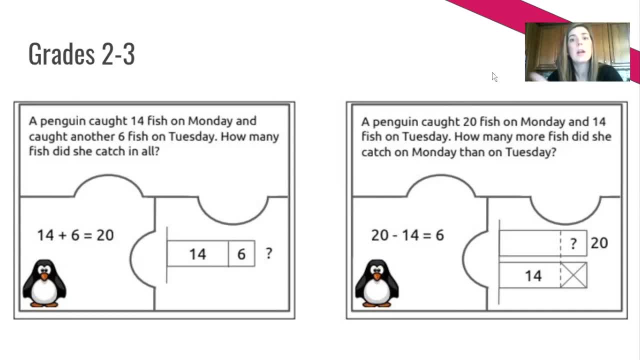 the part. We know the whole. We know one part. How do we find the other part? This one on the right hand side is comparison, because it's how many more They need to get used to all of that wording in their word problems. So again, our penguin numbers that we're working with. 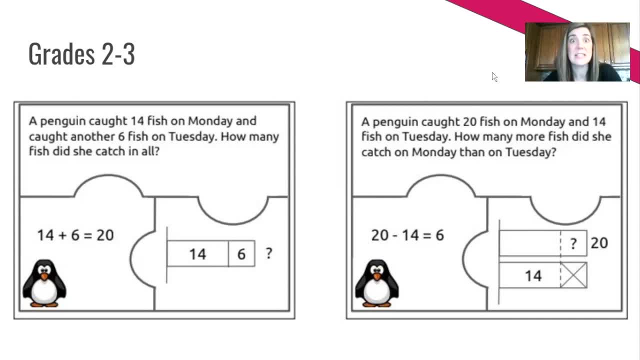 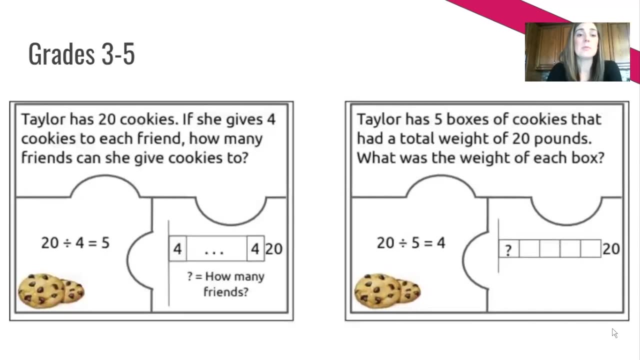 are 6,, 14, and 20.. So they cannot just find the numbers and put them together. The visual model has to make sense with the equation and with the word problem that they're given. Our next set deals with cookies. In these problems we're dealing a little bit more with multiplication. 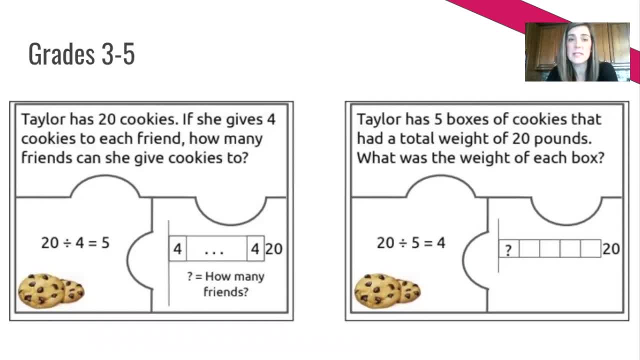 and division. There are still some part, part, whole problems on here. But it's also using our whole, knowing how many parts it's cut into, And then we're dealing with the whole. So we're dealing with the whole, knowing how many parts it's cut into. So how many are in each part, Or we know. 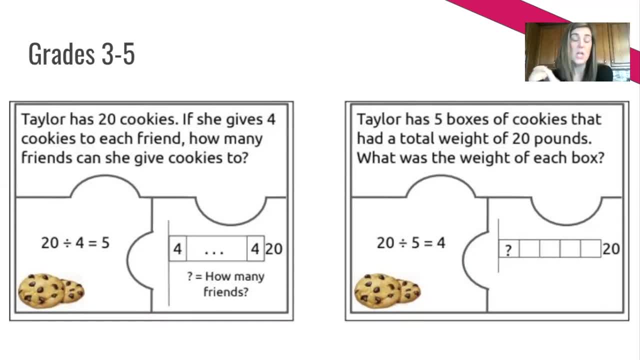 each part. We know the whole. How much is each part worth? So these questions have a little bit more to do with our multiplication and division standards that we have in fourth and fifth grade. Again, we're sticking with the same three numbers in the fact family 5,, 4, and 20.. 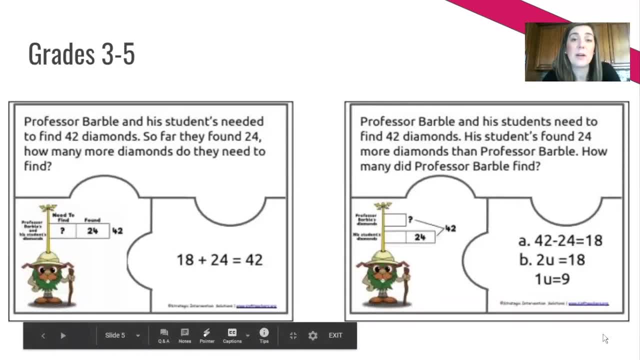 And our last set of puzzles deals with Professor Barbel, from our friend Shannon at SIS for Teachers. So Professor Barbel is going on a diamond hunt with a student. These problems are more for our third, fourth and fifth graders, because you'll see the problem. 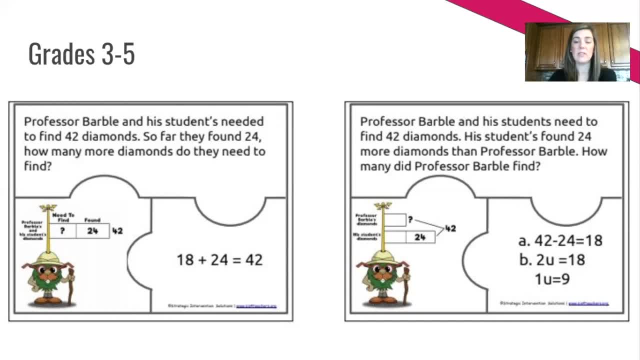 on the right-hand side of the screen. We're dealing with having to figure out what one unit is for. So first we're going to have to subtract the 24 from the 42, because his students found more diamonds than he did, And then we're going to have two units that equaling that 18 that we took the. 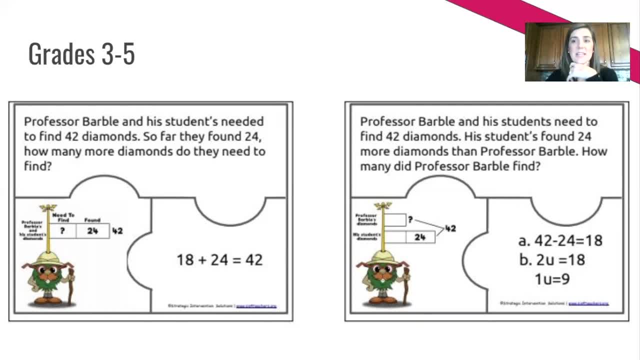 24 from the 42 to get, And then we have to divide that out to get how many are in one unit, So multi-step problem. So each of our set of puzzles have six puzzles on them, So you copy those puzzles onto cardstock. 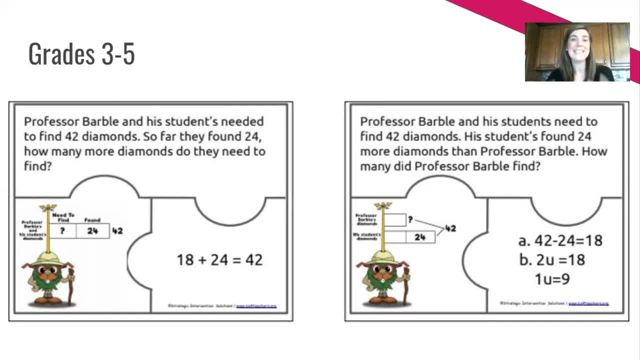 You laminate them, You cut them out, You put all 18 pieces for each set in a baggie. You hand that to a group of kids or a singular kid. I like to do it in groups so that they can collaborate and share their thinking and work through the problem together. And then the kids go at it and you come. 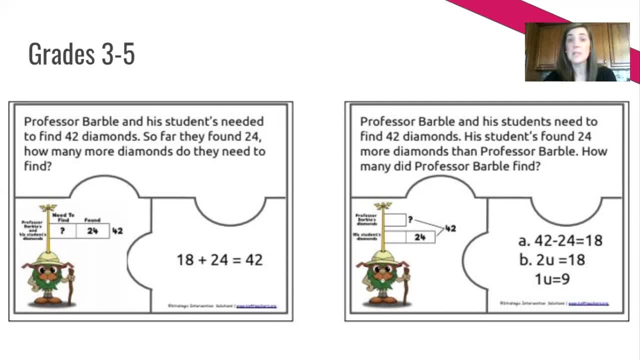 over and check And you might say: oh, you have two complete puzzles. Don't tell them which puzzles are correct, Just tell them how many complete puzzles they have and then they have to go through and analyze each puzzle. Another way to do visual models besides just doing puzzles. so kids aren't drawing those visual models. 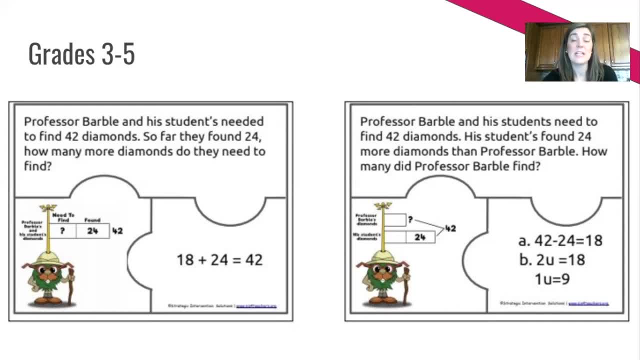 all the time is having them build the visual models with Cuisinart rods. I do that a lot. Cuisinart rods are one of my favorite favorite tools and my kids love when I give them a break from drawing visual models and they can just build it with their Cuisinart rods. But they have to. 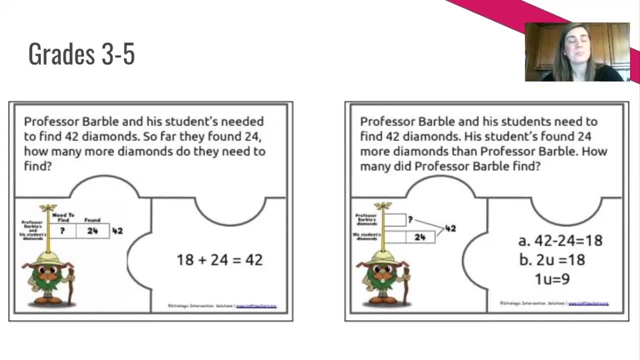 explain to me why they chose certain Cuisinart rods, certain colors, And it's that thinking that allows me to really know if the students understand and at what level. Another thing I use with more of my primary kiddos when I'm working with them are Unifix cubes, So I allow the kids to build with 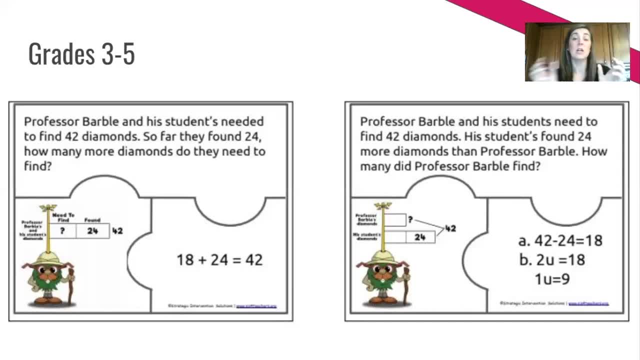 Unifix cubes, building those visual models, bigger or smaller, using different colors. Continuing to get that concrete pictorial abstract is huge. So this is just another way, using these Cuisinart rods, to see if kids have an understanding of what the problem is explaining and asking. and